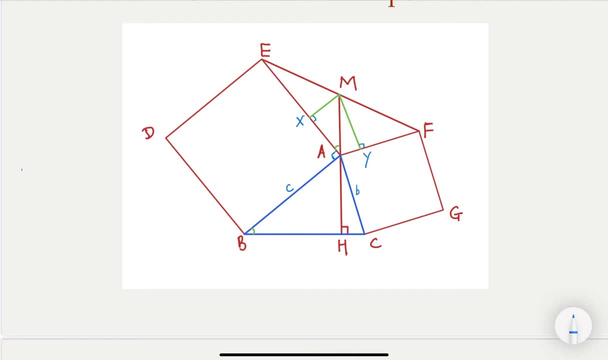 perfect applause. Create right. This is a C. This is B. Everything here is a square. This is C. this will be C. this will be c. this will be c. Alright, that's good. Now let's see the green angle here and markers on one, The other one and Mark it's a three, And I mark this angle is two. Alright, so notice that two and three add up to 90 degrees. That's fair clear, because in the red triangle two and three add up to 90 degree. But how about? 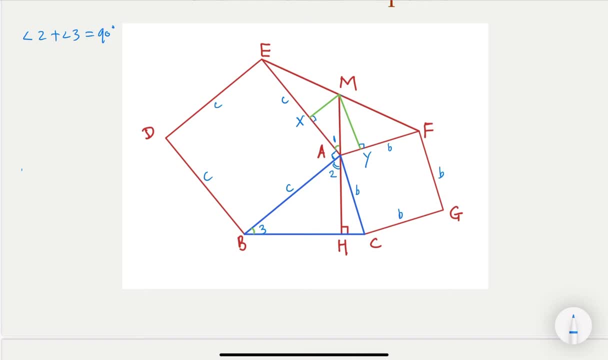 1 & 2, because 1, 2 and this right angle here add up to 180 degree. of course, in that case 1, 2 plus 90 degree equal 180 degrees. so if you cancel that's equal to 90 degrees. so from this two equation you know that 1 equal to 3. now here let's. 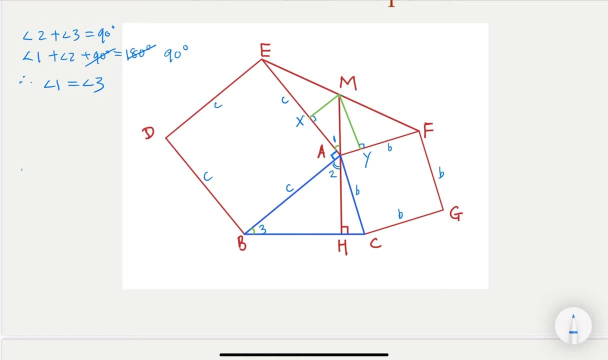 look at two triangles that are similar because they're they're right angles, and 1 equal to 3, so this angle here and then this market here and that one. you know, the two are similar, right. so with that, the corresponding sides are proportional, so let's mark them right. so I'm going to erase the marking here, right, and we? 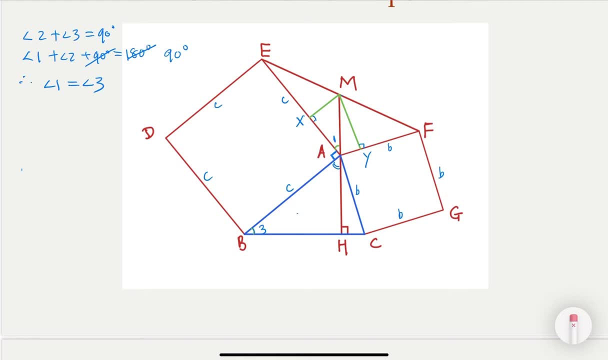 raise the marking here. so what the size I'm interested in is. let's call a H, let's cut it says edge, and then let's call a M. let's call this says M, and let's call this X. let's cut this way. okay, so that. 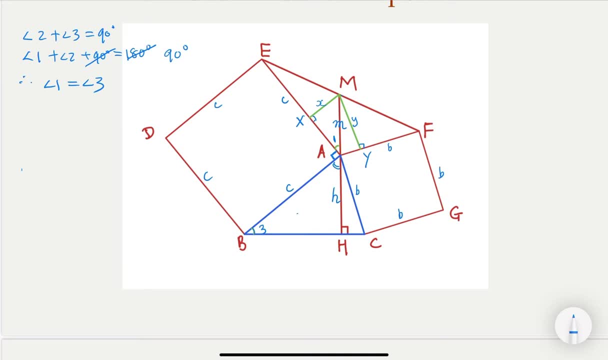 the length of the segments, right. so since two triangles are similar, as we mark earlier, so its corresponding says here I am interested in H and C from triangle a VH, right, so a VH is similar to axm, yeah, so here i'm going to have the size, and c and h the corresponding one. 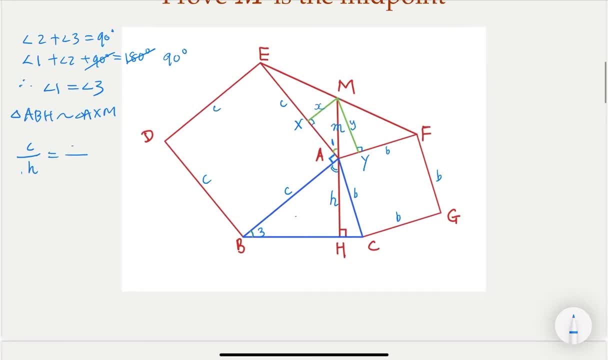 and the corresponding c would be m, right m and x. all right, that's good. now, similarly, on the right hand side, i claim that if you look at this, this triangle and and the other triangle use a similar argument. they are similar- and then use a similar argument. you know that the corresponding size 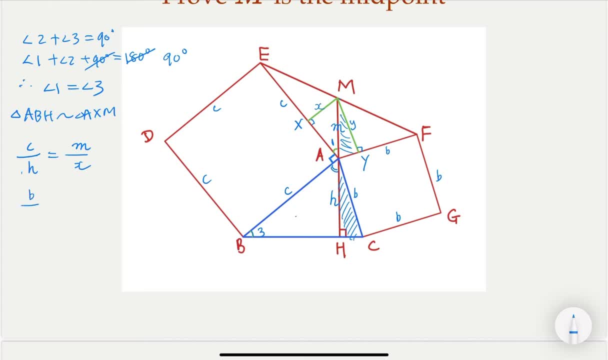 in this case h and b. b and h must proportional to, and here would be b and m, right, so, oh sorry, not b and m, and this would be y. okay, yeah, y and m. yeah, so would it be m and y. yeah, so it's corresponding now from these two, you know. 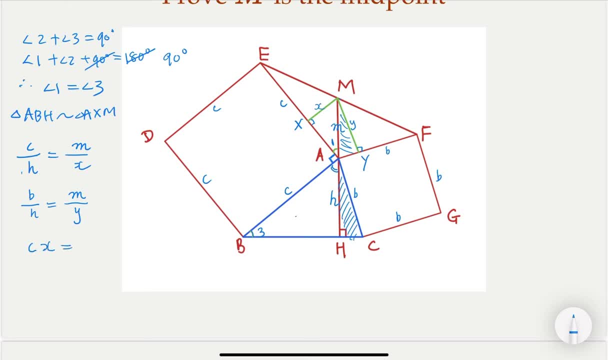 that cx equal to. from the first equation, cx equal mh, but from the second equation, mh equal b times y. but okay, let's erase some marking here. let's look at what the meaning of this, right, so you notice that this is b. yeah, let's mark it. 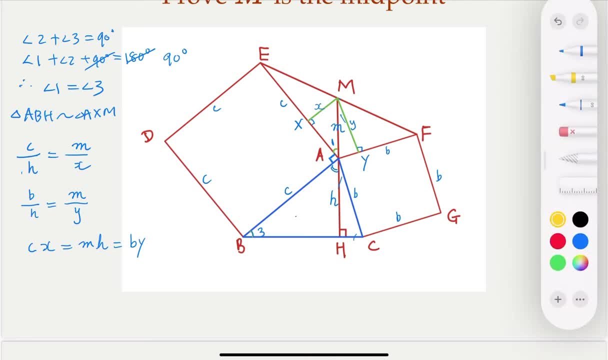 i'm gonna mark it with uh, with this one, so you notice that b, yeah, and y, yeah, by here would be the travesty of the area of triangle AMF. yeah, so BY here. this is, let me write it here. so BY here. this is 2 times area of triangle AMF now. similarly, when you look at C and 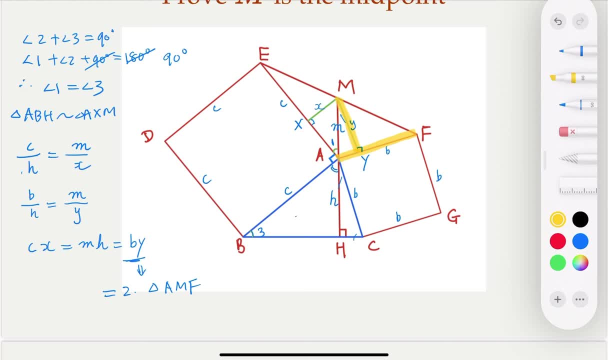 X. right, let's mark it again. this is a C, yeah, and this is X, so it is a triangle AME, yeah, so you could try some triangle AME. so, all right, I'm gonna erase that marking again. so what we're saying here is that: the triangle here. 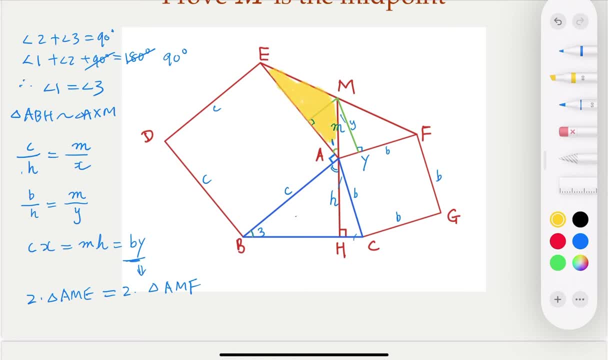 yeah, this triangle and change the color here and the other triangle, yeah, they have same areas. so in that case, I claim that M is a midpoint. in other words, M E equal M F. you may wonder why that is the case, right? so if I have a triangle here, yeah, 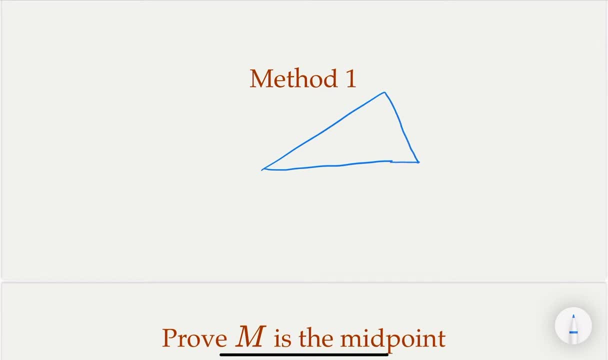 yeah, yeah, let's say M here. I have such that this is E and F, right. so experiment. OK, is going to be this one, this is going to be the height, this is going to be edge, and the right hand side, the height, is also edge, right, so the the same, then the. 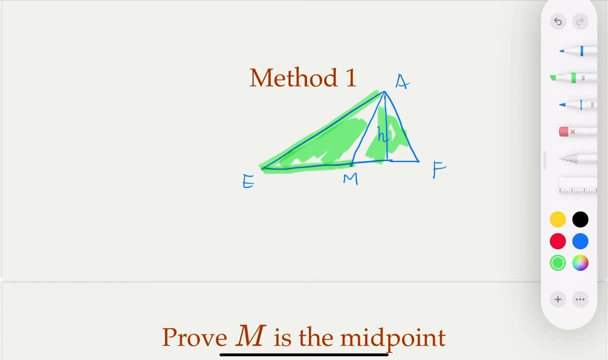 two base must equal to each other. in this case, two base would be would be one. one is this place, the other one is going to be that base. so this M is going to be the midpoint, right? so we prove it. this is a matter number one. all right, so let's. 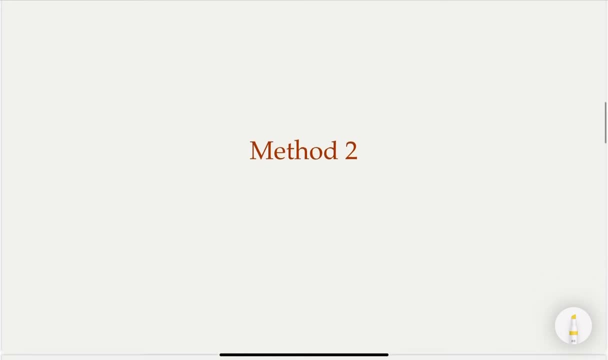 go to method number two. so in the method number two, what are we going to do is I'm going to construct a line parallel to a edge from point E, okay, so this is going to be parallel nine, yeah, parallel nine, yeah, to A edge. okay, but I'm gonna let this line meet with. 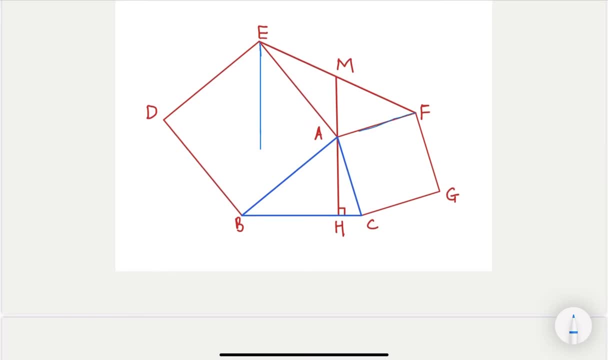 the extension of A F. okay, So I'm going to extend AF here. yeah, and this line meets at: let's call it G, right? Oh, sorry, G is used, So I'm going to call it. yeah, I'm going to call it T, all right. 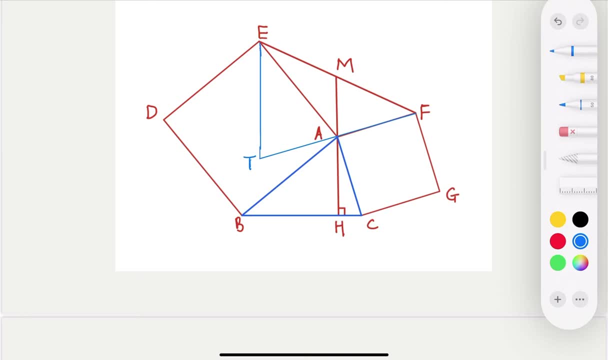 Okay, so here I claim that I have congruence triangle now. Now can you spot it? congruence triangle here. So remember ET, parallel with MH, right. And I claim that the triangle here, first of all the sides, this is a C, this is a market right. 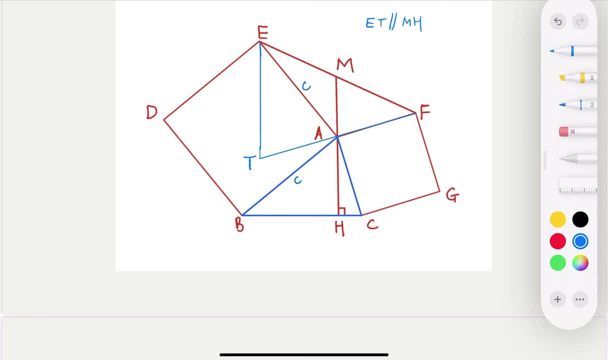 This is a C here. Okay, that's good news. So I have, I have one side is equal to each other, right? And since I have this angle here, let's look at this angle here, right? Yeah, so this angle is actually 180 degrees and let's call this is the other angle. 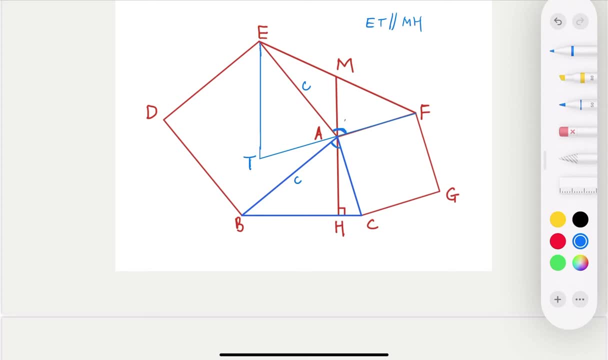 I claim that they complement each other, right? So if this is angle 1, this is angle 2.. So I claim that 1 plus 2 equals 180 degrees. Why It's? because the other is 90 degree. This is 90 degree and this is 90 degree, right. 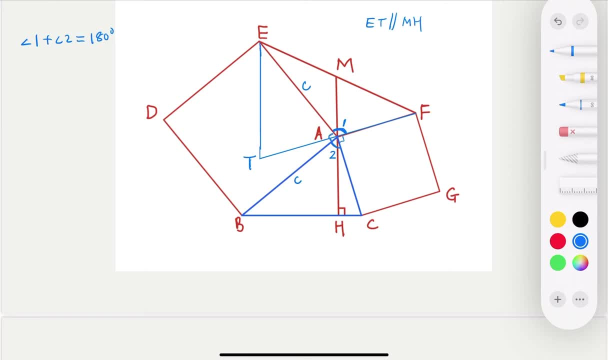 So the full circle is 360 degrees, right, So 1 to 180 degrees, Okay, so here, but when let's erase this here, this is 90 degrees. However, you notice that this angle here, yeah, complement of 1,. 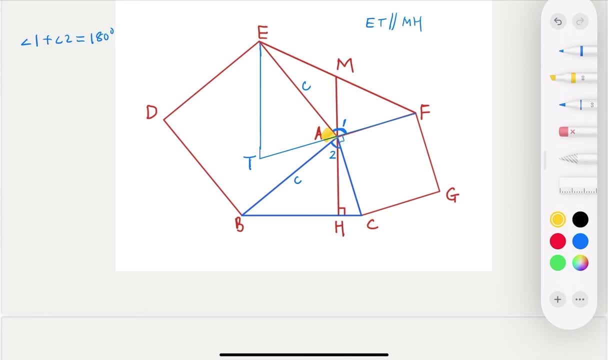 it's going to be this one right. So this triangle here, this angle here, yeah, let's call it 3, right. This is angle 3 here, equal right. So, in other words, 1 and 3 add up to 180 degree. 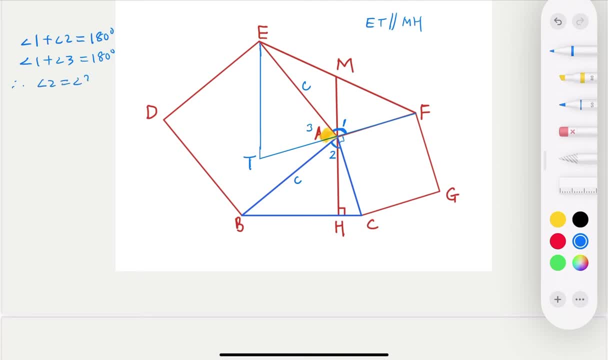 So 2 and 3 equal to each other. okay, So I claim that the two triangles are congruence. okay, I'm running out of color, but Let's mark them. One is ABC, the other one is this triangle here. 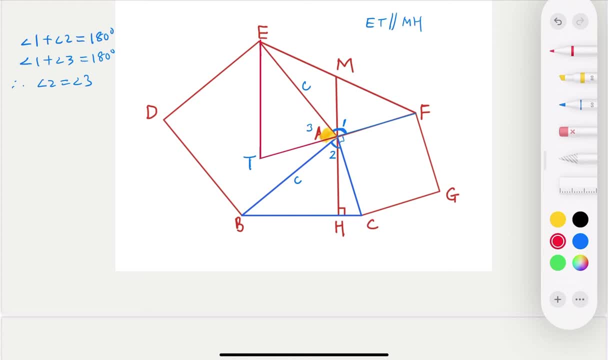 Yeah, so one size is equal. This angle equal, right 3 and 2 equal. I just need to find another angle that are equal to each other, right? So let's do that. How do we find that? Okay, 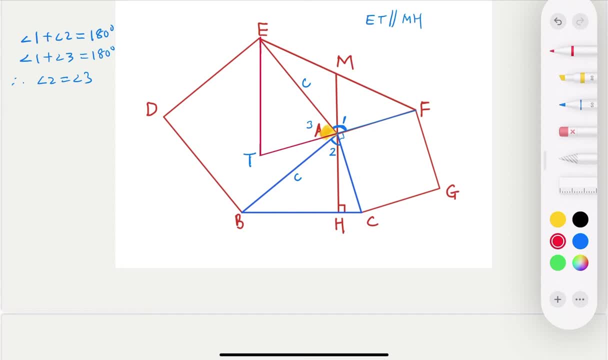 So here. So here we're going to use an easier way, yeah, Okay. So here, for example, this angle: right, Let's call it 4,, right, That's 4.. But 4, because this line is parallel, right. 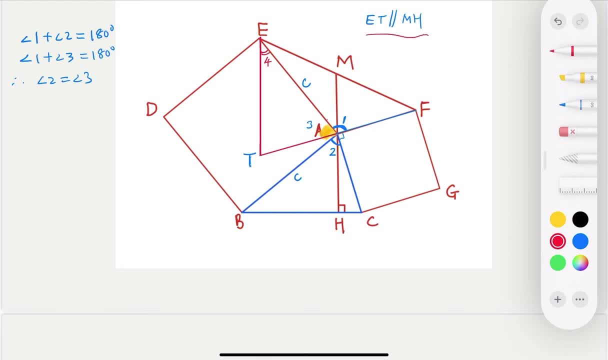 ETN parallel. So must equal to equal to. I call this 5, right. This equal. This is equal to 5.. 4 equal 5, right. So let's say that 4 equal 5, yeah. 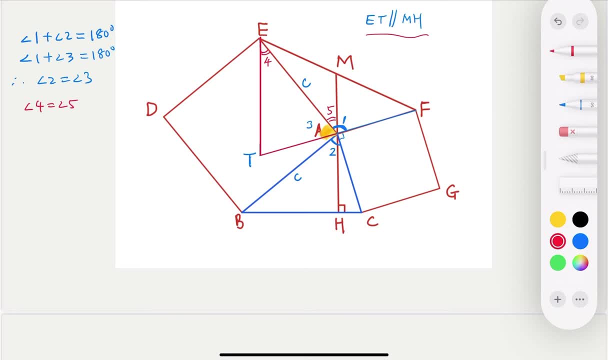 And for the 5,, when we think about it is there is a 90 degree here. right, This is 90 degree here. So let's call this angle here, yeah, This angle. let's call it 6, yeah. 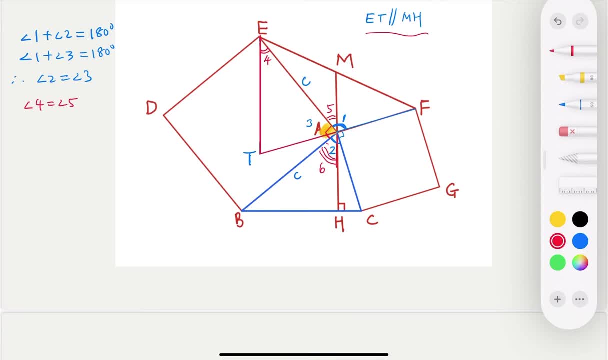 So 5 plus 6,? yeah, So 5 plus 6 equal 90 degree, And 6 plus 7 is 90 degree. yeah, 7 plus 6 is 90 degree. So what do you have? You have, 5 must equal to 7, right. 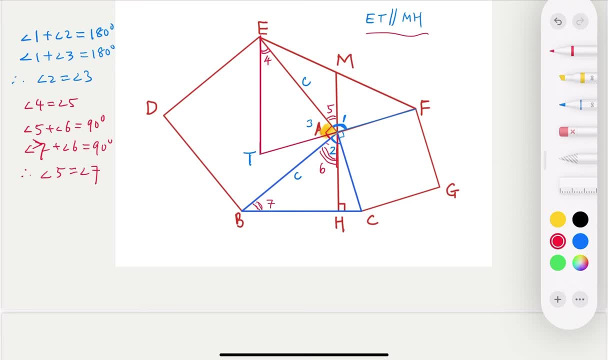 So 7 equal to 5 equal to 4.. So this is 2 triangle. I have 4 equal to 7.. I have earlier, I have this triangle, this bigger one, number 2, right Equal number 3, yeah, 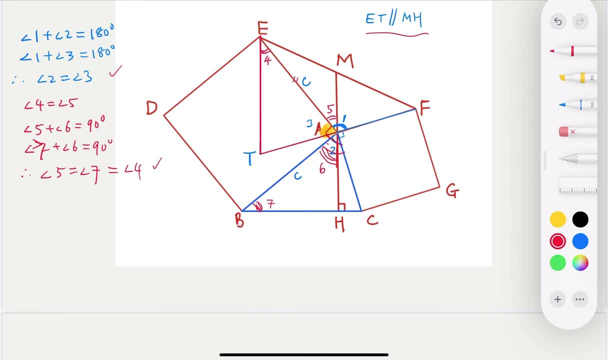 4 equal 5.. And the size equal here. This is C and this is C. So I say that triangle ABC is congruent, right, ABC, yeah, Congruent with AET, Okay, Okay, Yeah, So when they are congruent, what do you can? 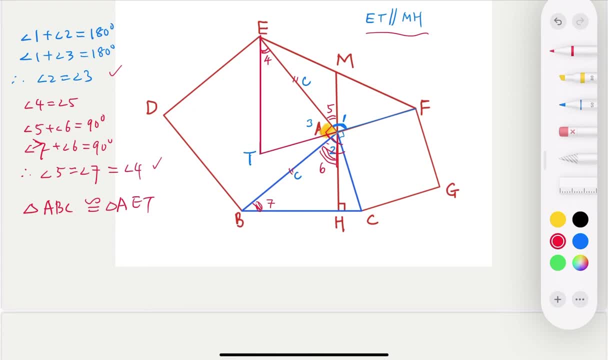 Know, is that this one, yeah, must equal to the size here. let's call it the B, right? This must equal to B, But then this is also a B, yeah, Because so, which means you have- let's look at the big triangle here. all right, 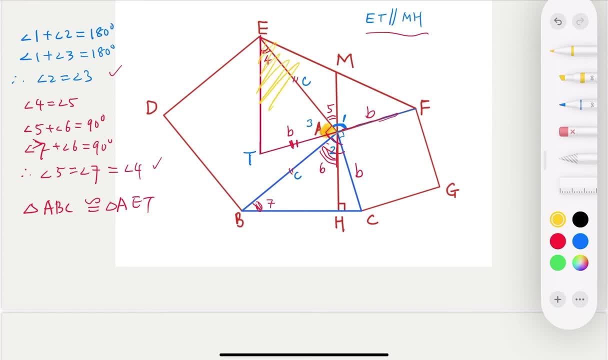 Let's look at this big triangle here. Oh sorry, Let's erase it. Okay, Let's look at this big triangle here. right, This big triangle. yeah, I have this B equal to each other, right, Okay? So this is going to be midpoint. 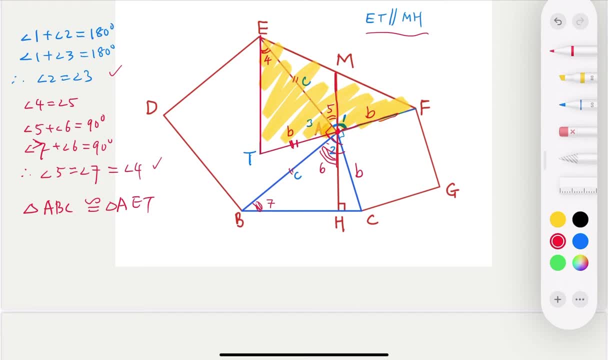 This is a parallel line- yeah, Parallel line- of this. Since this is a midpoint, of course, the other one must be also a midpoint. all right, So we just prove. Prove that M E equal M F Y, because A T equal A F. okay, 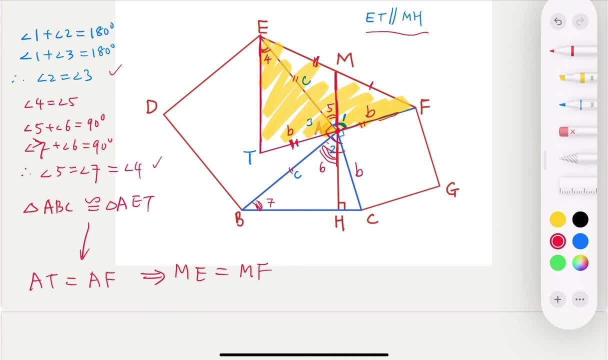 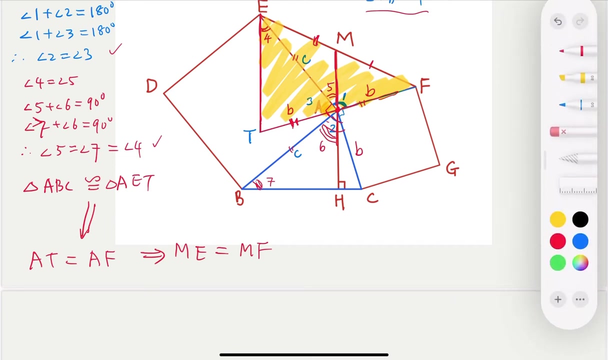 And because they're congruent, right. So that's it. So that's kind of the second method, all right. So hopefully you follow the steps. You can pause the video and think about the steps, all right. The key step is actually try to prove that these two triangles are congruent here, right? 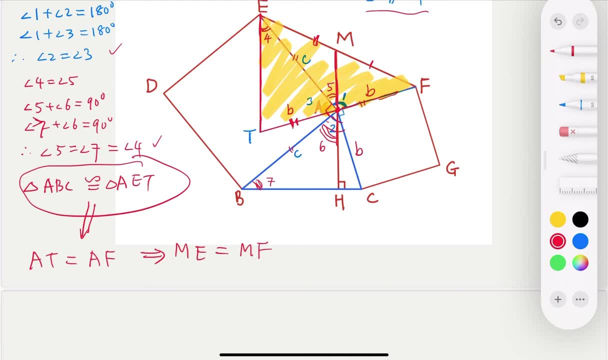 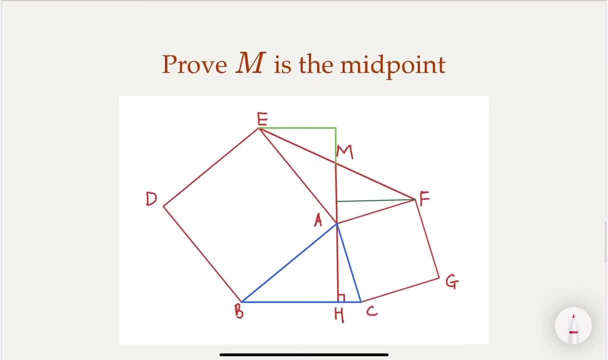 So here, that's the key for method number two. Let's move on to method number three. all right, So it's all about how to construct. you know some special line for you to prove. What do we want to prove? 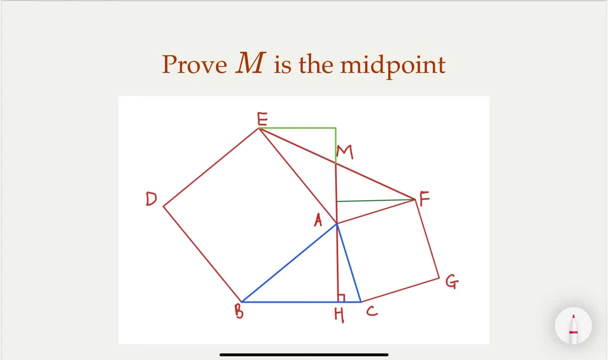 Here we're going to also do a perpendicular line, but this time I'm going to from E and from F, right From E. I'm going to try to do a perpendicular line here. Let's call it this X. Let's call this Y. 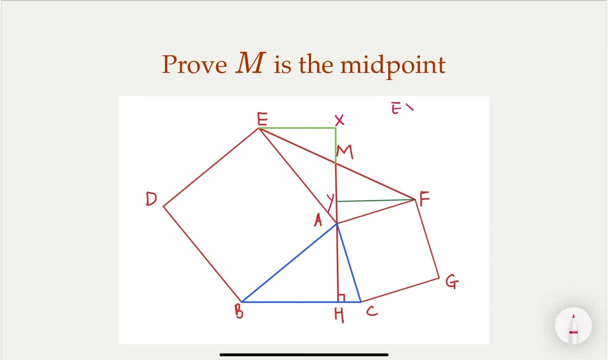 So I'm going to have EX perpendicular to, you know, this line HM And we have this FY perpendicular to this line HX. Of course, in that case they're parallel right. So I claim that the triangle are congruent. 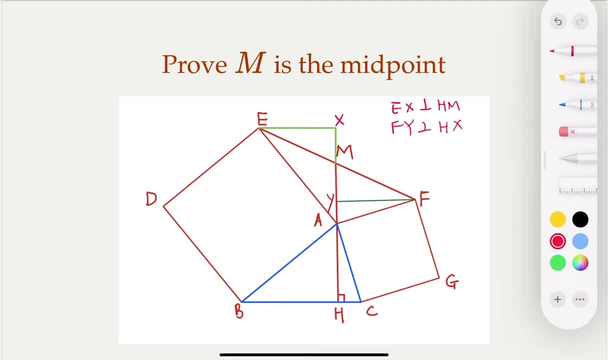 If they're congruent, then I prove that. the ninth segment is, you know, midpoint, right? So how do we do that? So we want to prove this right: triangle are congruent. yeah, So which two triangle are congruent? 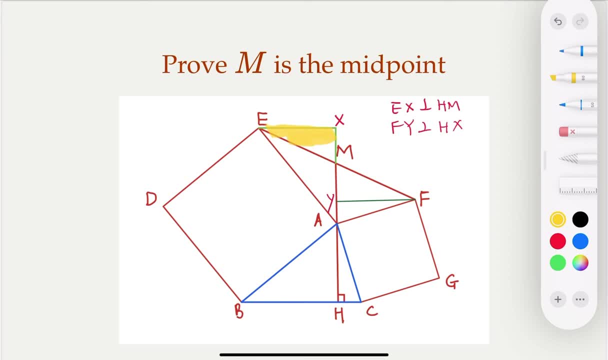 So we want to prove this one here. Yeah, And this one are congruent, yeah, So of course you, because those are right angles here. yeah, You just need to prove maybe one side equal to each other and this angle equal to each other. 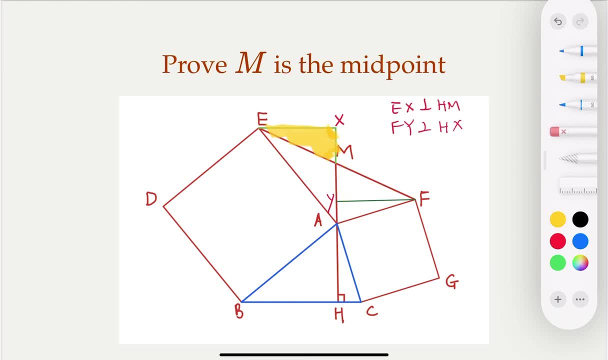 So let's erase that, Okay. So how do we prove one side's equal to each other? In other words, if we can prove ex equal to fy, then we're done right. so here i claim that i have a congruent triangle here. 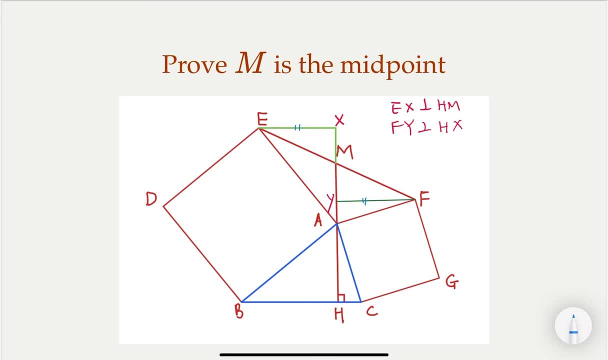 and that is, and i'll claim that triangle f a y, yeah, f a y is congruent to a, c, h. okay, why, first of all, this right hand triangle? right, and then the size is equal to each other. right, because if this is b, this is also b, and the angle here, this angle. 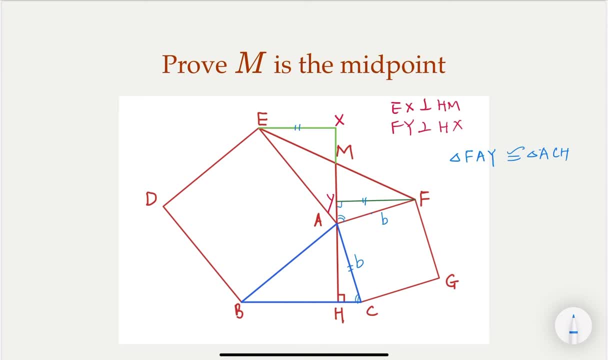 yeah, is equal to this angle. similar argument earlier. right, this is one and two add up to 90. three, this is three. yeah, this is like one plus two equal 90 degrees and the two plus three equal 90 degrees. so one must equal to three, and then the two triangle are congruent. 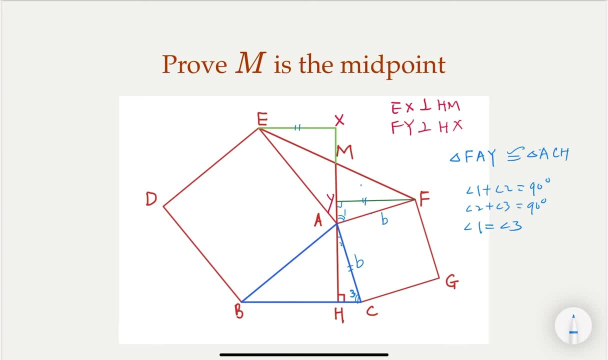 so this one was equal to b. all right, so we got it. okay. so, and now we need to prove ex equal to b. all right, oh sorry, it's not a, b and this is not. this is not b. the z is uh- doesn't answer the mistake- and this is ah, which is h. right, this squared. 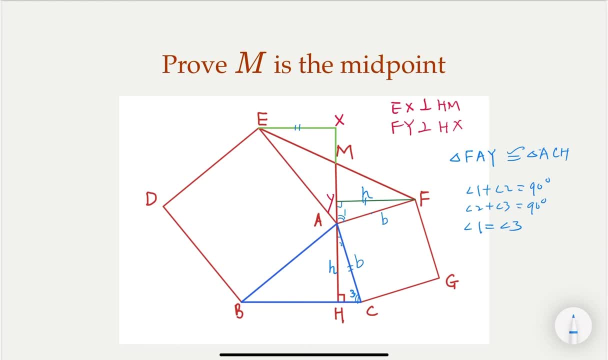 h. okay. so fy, yeah, equal h. we're going to prove that this is also h. so how do we do that? i claim that i have two congruent triangles here. then this is also h. right here, an earlier Tamil斔. so this is an earlier Tamil斔. how do we prove it? we're going to prove that in otheroko. so this is also an earlier Tamil斔. this is also an earlier Tamil lantern, then we need to prove that in other book. this is also a shall share in ch tape. oh, so i claim that an earlier Tamil lantern. 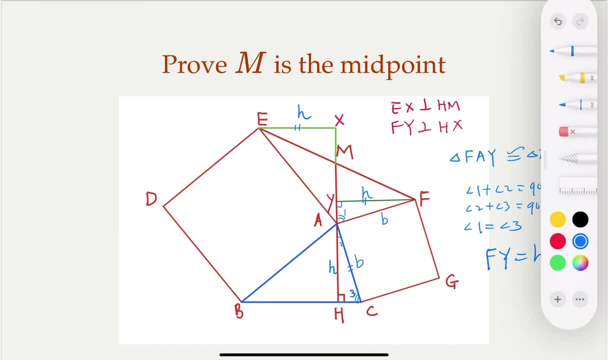 triangle here and mark them as green. okay, so one is this triangle here. somehow it doesn't work. yes, maybe mark like that. this is better, right, so this triangle here is congruent with the this triangle here. yeah, why? similar argument as earlier, right? so one is that if this length is C, this is also C and this. 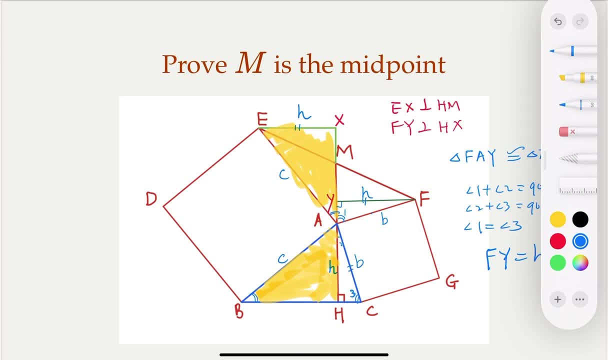 angle here equal, that angle here, right. so we're done. why? because this is edge, indeed, this is edge, so these two angle equal to each other, and then let's erase this. yeah, so now I have this triangle, a congruent with each other. also, right, because they. 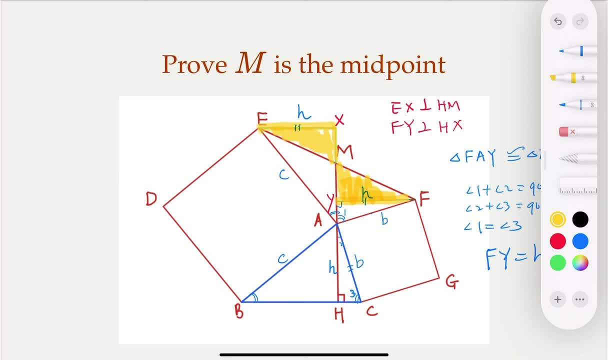 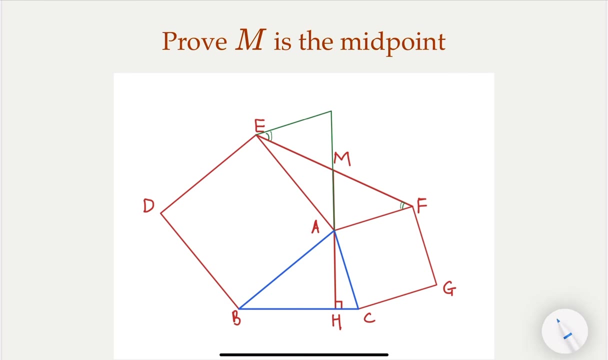 have common, common ends and the red red angles. okay, so M is a midpoint, right? so that is that. this is method number three. now method number four: all right. so you find it interesting that there's so many ways to prove this right. so here, what we're going to do is we're going to use this method number three and we're going to 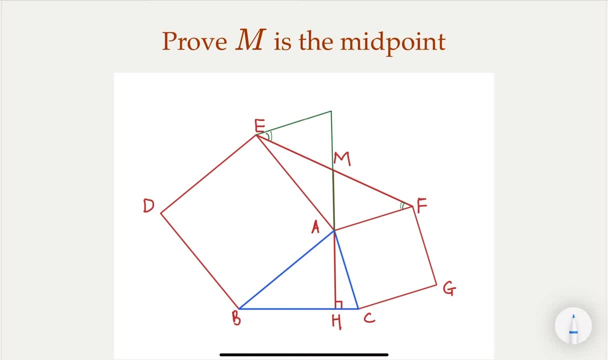 do is we're going to use this method, number three, and we're going to doing here, we're gonna construct a parallel again square this X, so we're gonna construct ex Imperial to AF, yeah, and I'm gonna extend a match, and then intersection point is: you know, this is just or write, so we want to. 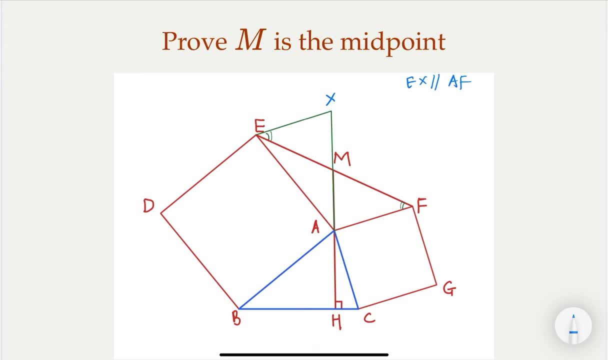 prove having a friend group unless you аs Go ahead now. let me think I didn't echo image of the Nana weak me, you know it at all okayfish into a unit. pulls with the end M a match with the end M, a match with the end eif, at the end eif, I say- 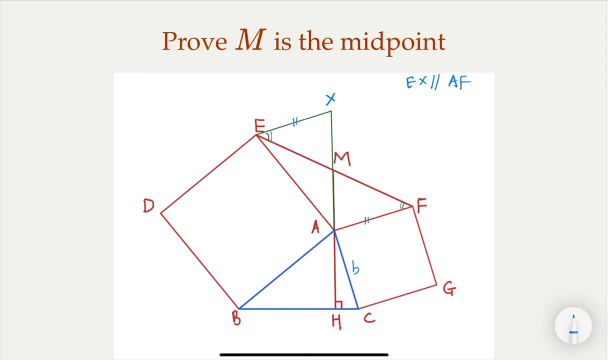 again. let's mark it. so the size here could be: everything is b here right, b here and here. this is the parallel line here. so the angle one must equal to this. angle one must equal to angle two, right? so how do we going to prove ex equal to b? i claim that i have congruence triangle here, right? so this time i'm going to 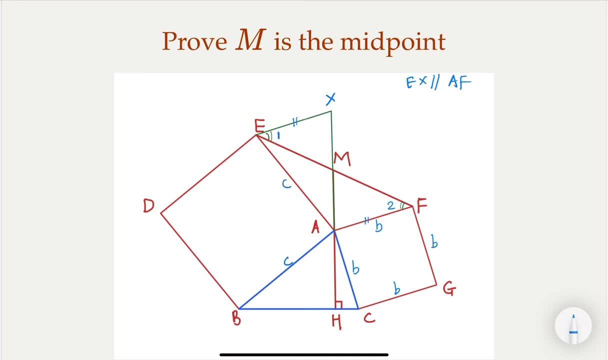 look at this c. okay, so i'm looking at abc. yeah, i'm, i'm going to look at this triangle here. let's mark it as a as here: this one, yeah, okay, so, okay. so this triangle here. i claim that i have one angle right equal to this. as earlier, i'm not 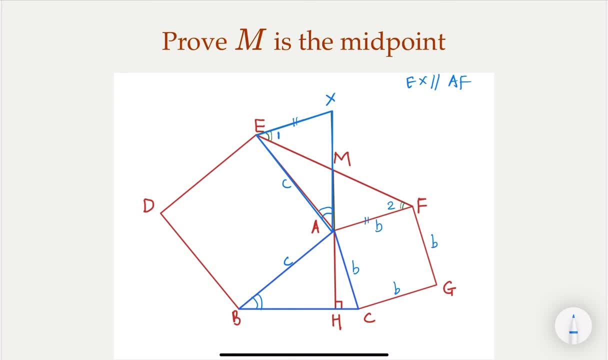 going to repeat that, yeah, i have size equal at this, size equal c. right, i have size equal c. and i have another angle here. let me see we need to prove it anyway. okay, all right, okay, okay, okay, let's go. okay, okay, okay, yeah, So, because this is a paradigm line, right? so what I have is: 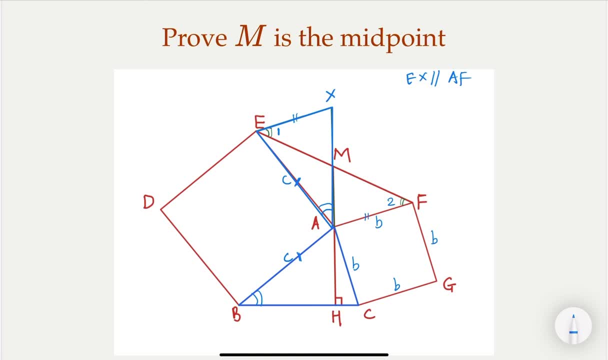 Okay, it's very easy. so this big triangle here, right, this big triangle here, yeah, let's call it Three, right, and this one is This: four. so three plus four equal 180 degree, because nine a parallel right. Three and four, this is four. now four and this. 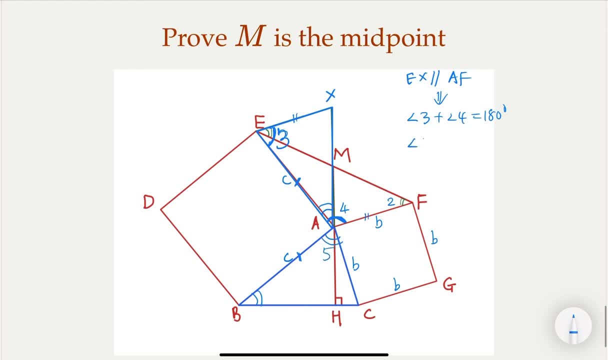 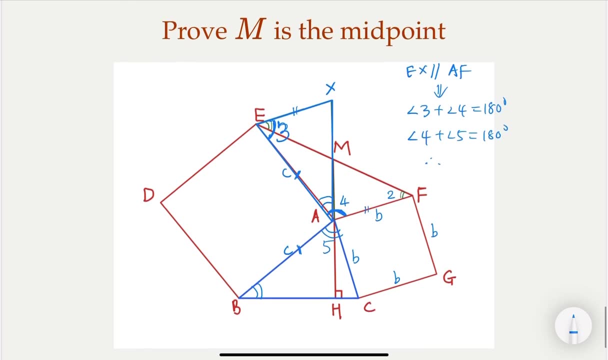 Yeah, let's call it five. so four and five is 180 degree. so in that case three must equal to five. Yeah, so I have one size and two angle equal to each other. So the triangle are congruence, in other words, ABC Is congruent to. 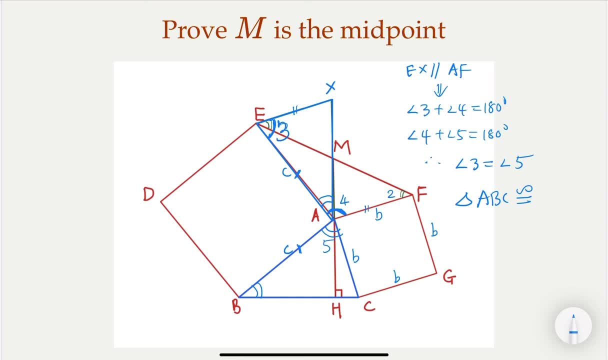 Yeah, so E a X. so in that case, e X must equal to AC, and that means, Because AC equal to B, right? So here, what do you have? so e X, You could be and must equal to AF, right, AF. So, since you do a parallel line and this, if you could claim that this is equal to each other. 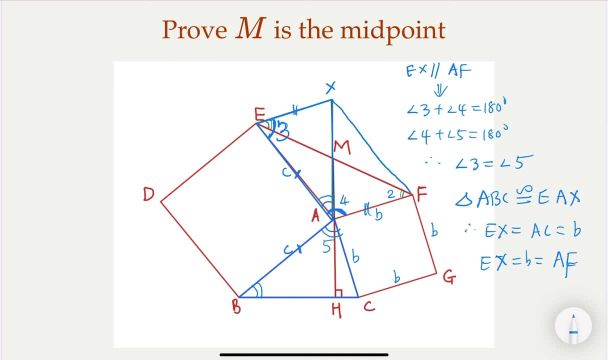 Then, of course, the this might be parallel. right, This is XF, Okay, So, So Am is the midpoint, because this is parallel. Somehow I couldn't connect the nine here, Okay, so when we look at this Shape here- So this is the midpoint- there's an intersection point. 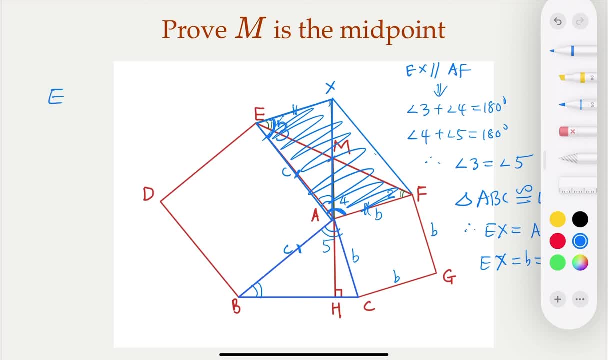 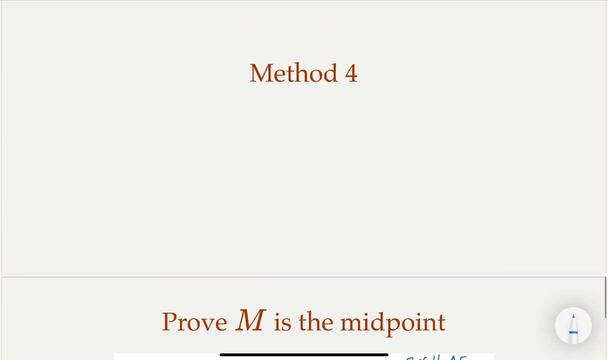 is going to the midpoint. so M E, M equal M F. right is because we have this parallel line and the size equal to each other. all right. so we presented four different methods here right of the original problem and hope you can follow the steps and, if you have yet another method of proving the original. 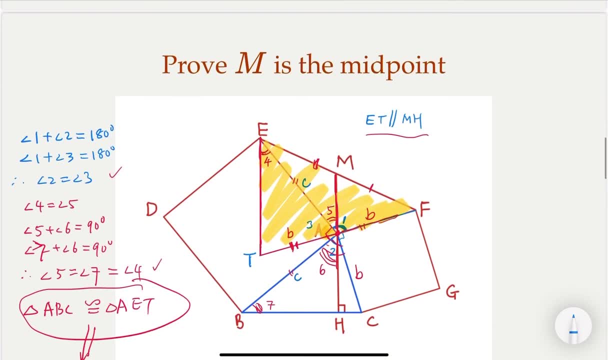 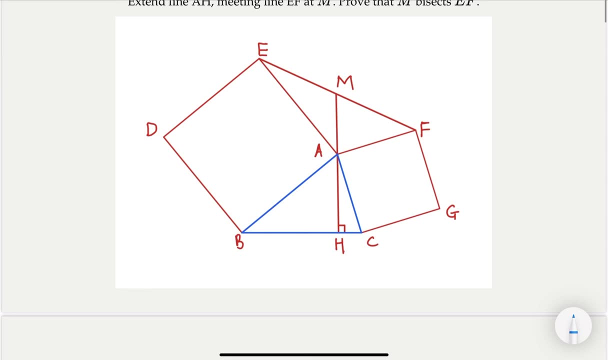 problem. I'm interested in and knowing your methods. please leave a comments below. all right, so this is the original problem and please subscribe to the channel and for you know some other interesting problems. all right, thank you.